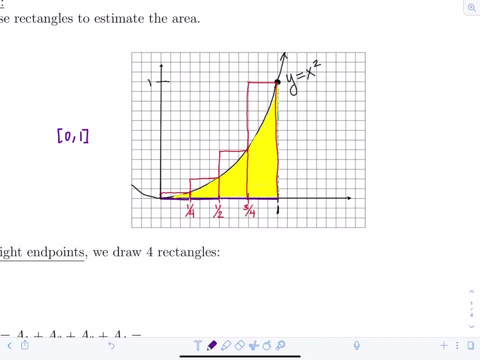 fourth, one, fourth, one, fourth. Now, the height of each rectangle is determined by taking the right end point of each interval. So if I'm breaking up the interval from zero to one into four sub intervals, I'm going to use the values on the right of each sub interval. 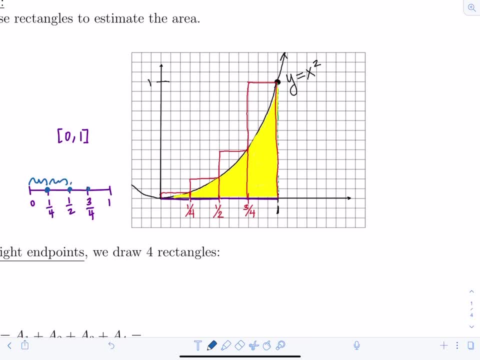 to evaluate the function. So one fourth, one half, three fourths and one. okay, And so the height of the first rectangle is given here by f of one fourth. So substituting in one fourth for x into x squared. The height of the second rectangle is determined by taking one half and plugging it into our 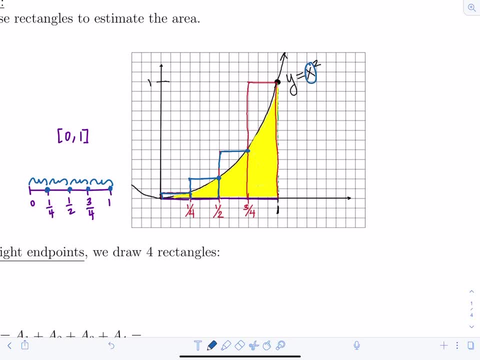 function. The third rectangle's height is determined by taking three fourths and plugging it into our function, And the last one is by taking one, the end point of the interval, and substituting it into our function. All right, Could we compute the area of each of? 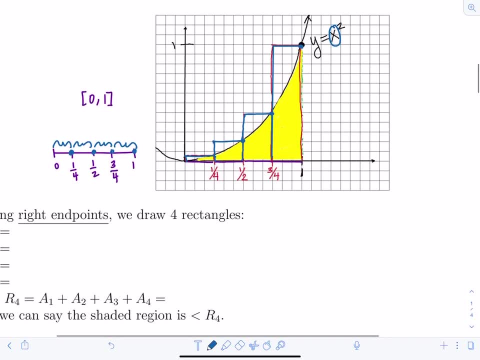 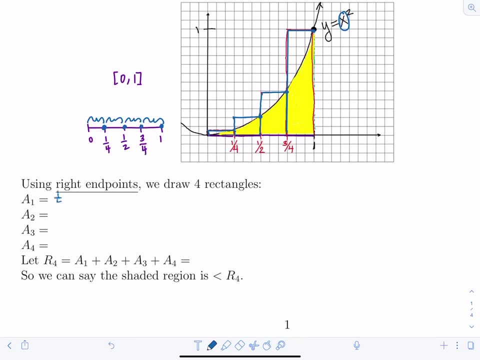 these four rectangles. Sure, So we have base times height. So the area for the first rectangle is going to be its base, which is one fourth times its height. Well, the height of the first rectangle is going to be one fourth squared. 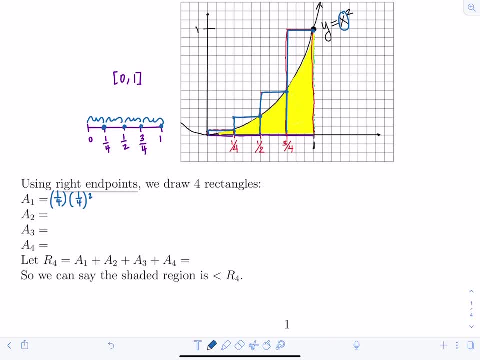 right, I'm substituting that into. y equals x squared, and the x value at the right end point of the first sub interval is one fourth. So this is going to give us one over 64.. The second rectangle's area. so this is a one. 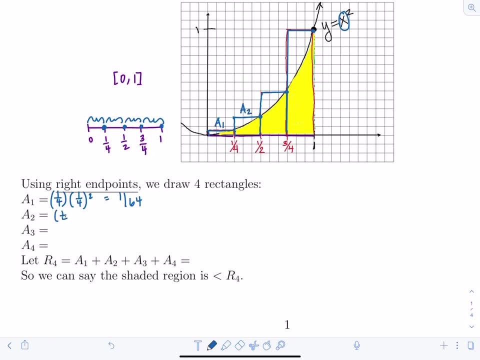 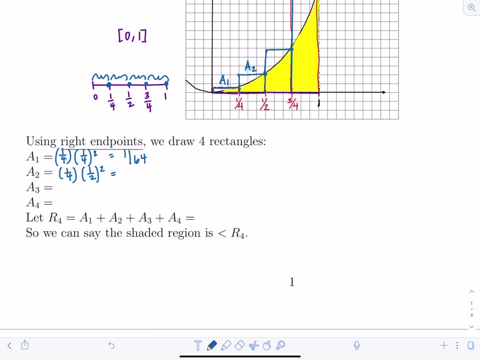 This is a two. Again, its base is one fourth. All right, Its height is going to be one half squared, So that's going to be one fourth times one fourth, which is one sixteenth. The third rectangle, a three, is going to be one fourth times three, fourths squared. 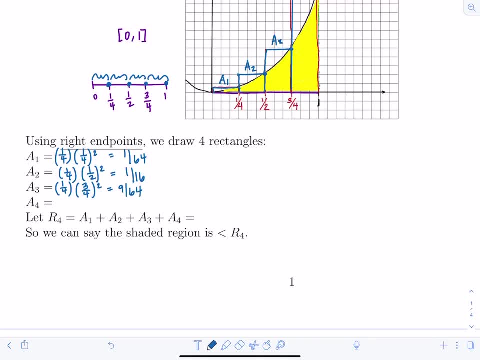 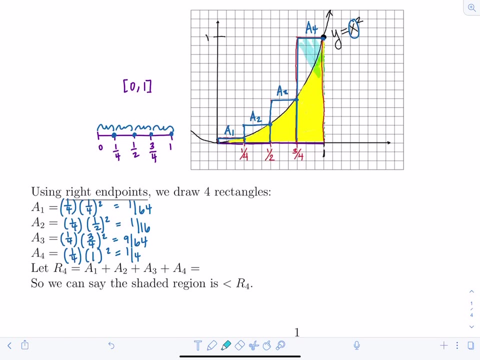 So this is nine over 64. And the last rectangle's area is one One fourth, that's its base times, one squared, which is one fourth, And here's a four. Okay, So let me highlight: Here's a four, a two, a three, excuse me, a two and a one All. 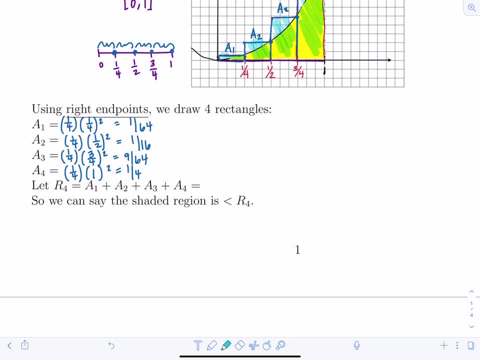 right. So we say r sub four, meaning the sum of these four rectangles that were made using right end points to determine their height is equal to a one plus a two plus a three Plus a four, And this comes out to 15 over 32.. So notice something important here. So the 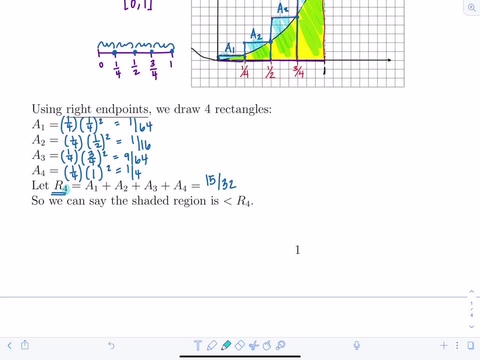 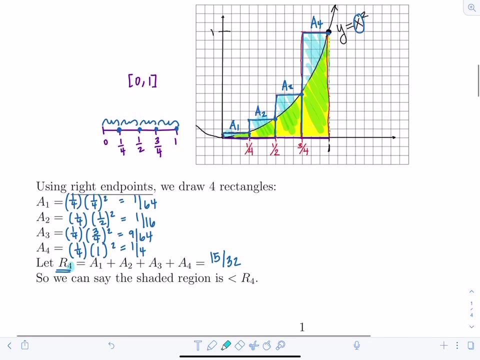 subscript tells you how many rectangles or how many sub intervals were used to create the approximation, And r tells us that we used right end points for each of those sub intervals to evaluate the height of the rectangle. Now let's look at the approximation that we have. r four 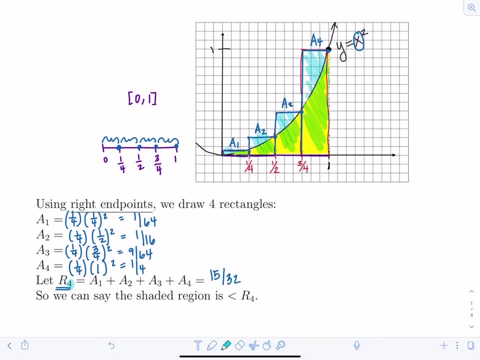 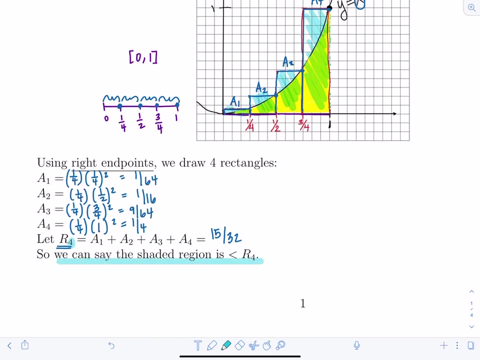 versus the true shaded area. We'll notice each of these rectangles lies above the curve. y equals x squared, So that means it's an overestimate of the true area. So we can say that the shaded region is less than r four right. So we know clearly it's not equal. 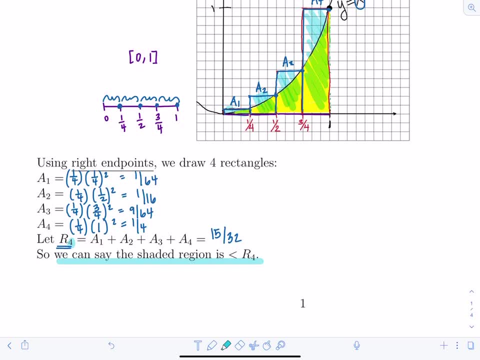 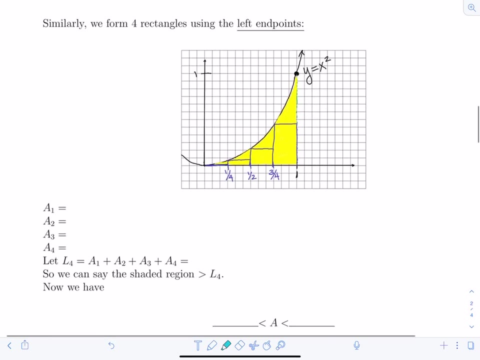 The exact area under the curve is not equal to 15 over 32.. It's going to be some value. less than that, Okay? Well, what if, instead of using right end points, we formed four rectangles, but this time we took left end points to determine the height of each of the rectangles? So here let's. 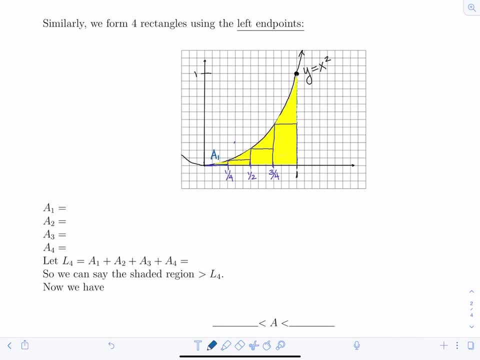 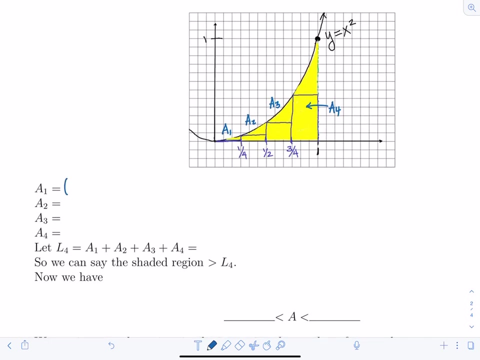 go back and label in: This would be a one, my first rectangle a two, a three and this one right here is a four. Okay, So the base of each of them is still one. fourth, So a one. a one's area would be. 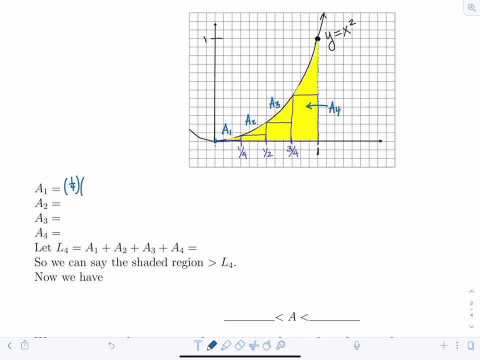 one fourth times. Now the left end point on the interval from zero to one fourth is the x value of zero. So I would substitute zero into my function. And the first rectangle has an area of zero right. You can see there's no height to it. Now the second rectangle's height is determined by: 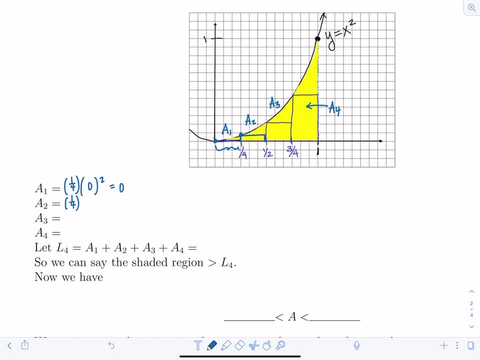 taking that left end point of one fourth. So I would have the base of one fourth times one fourth squared right, Because my function is y equals x squared And this is going to be one over 64.. All right, A three is right here, So base is still. 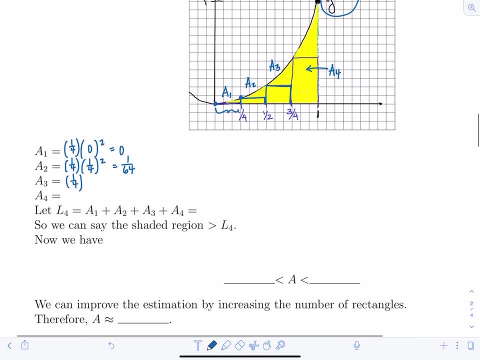 one fourth. Height is going to be one half squared right- See the left end point here. So this is going to be one fourth times one fourth, which is one 16th, And then a four base is still one fourth. The height is going to be determined by taking three fourths. 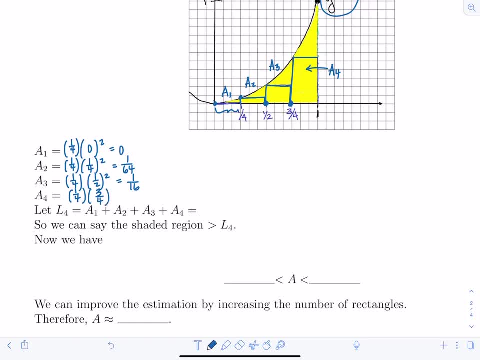 substituting it into the function. So I have one fourth times three, fourths squared, which is nine over 64.. Okay, So now we call this a four. So I'm going to take a four and I'm going to take a three. 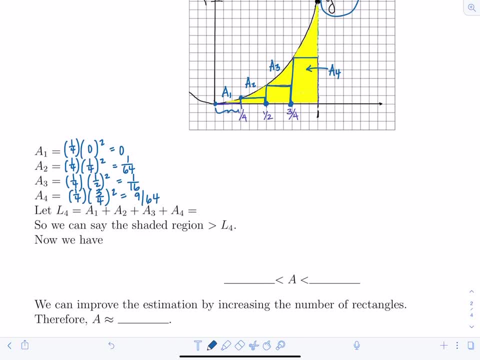 and I'm going to call this the sum of these four rectangles: L four- L standing for the fact that we use left end points from each subinterval to determine the height of the rectangles. and four, because there were four rectangles And this comes out to seven over 32.. 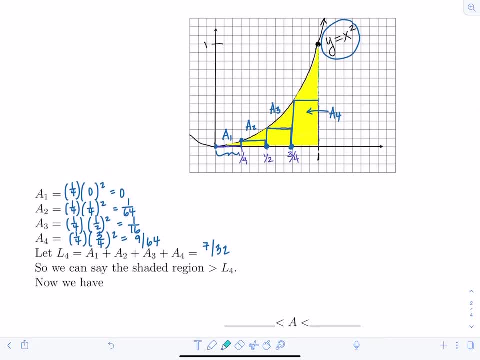 Now let's look at our approximation versus the true area. So here's a four, a three, a two and a one had no area. So would you say that L four, in comparison with our original curve, does a good job? Well, we don't know that. 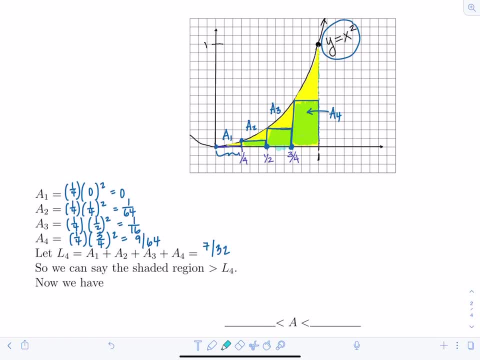 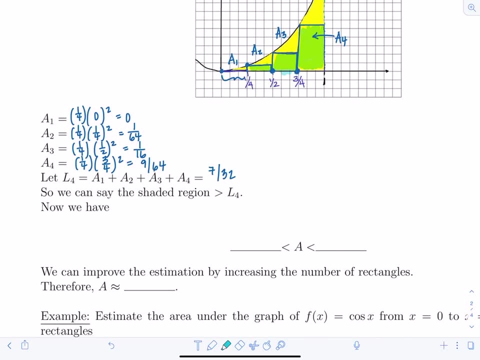 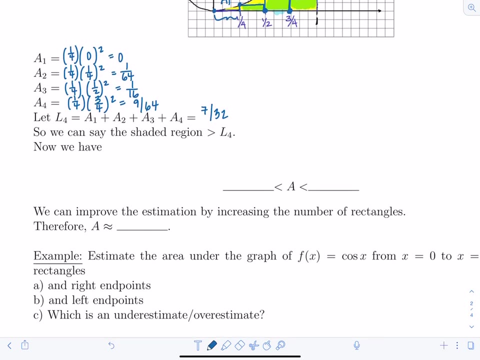 but I do know that it's an underestimate right. The true area under the curve is greater than seven over 32.. So now I can bound the true area underneath the curve. I can say that the true area, our last estimate, R four, was an overestimate. So the true area is less than R four. 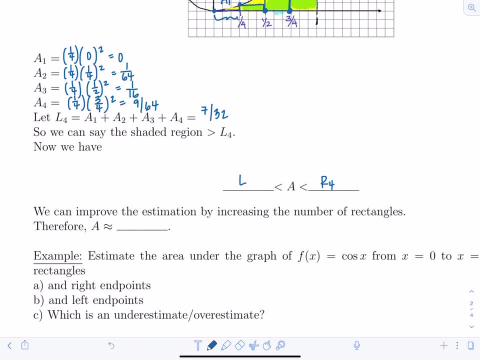 and it's also greater than L four, Something in between seven over 32 and 15 over 32,, but that's still causing quite a bit of room for error, right? So how could we improve our approximation? Well, what we would do is just: 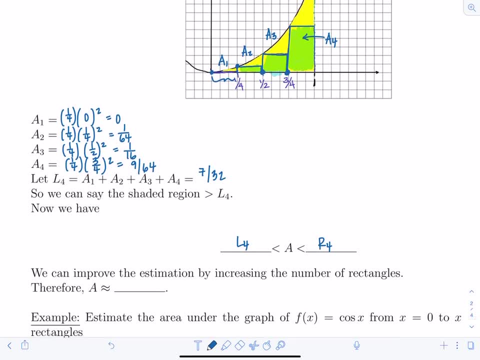 create more rectangles, right. Why are we only making four? Why not make eight or 16 or so, on and so forth? Then we would have less of an overestimate or underestimate by creating more and more rectangles, And that's the idea that we're going to build upon in the rest of the 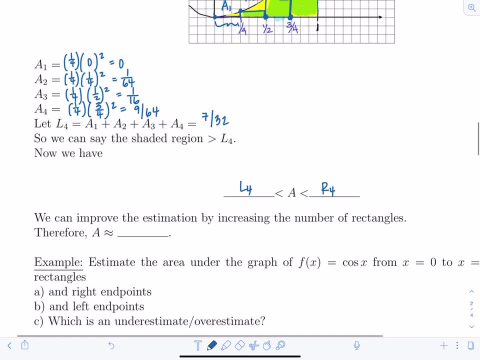 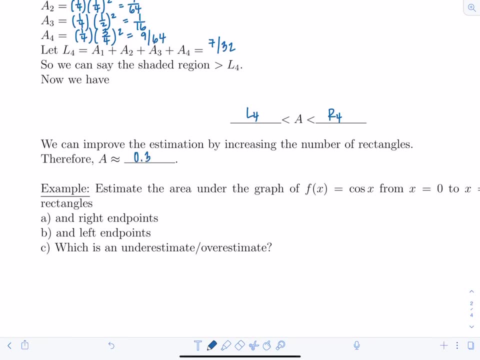 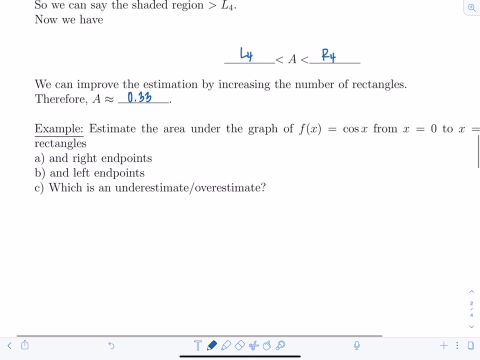 lesson, And later on we're going to show that the area underneath the curve is actually closer to 0.33 or one third. Okay, So let's practice using rectangles to estimate areas under curves for now, And then we're going to work on improving our estimate. So first we're going to consider a 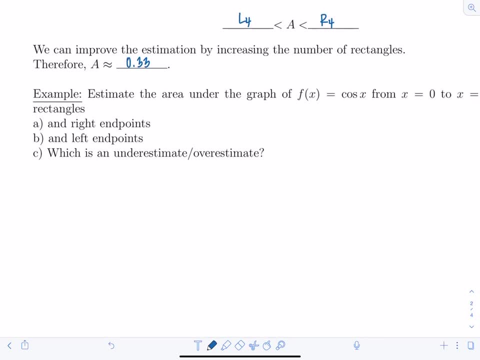 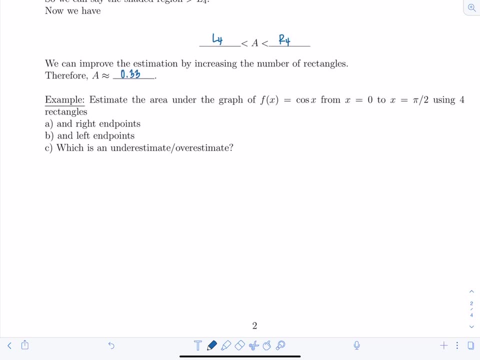 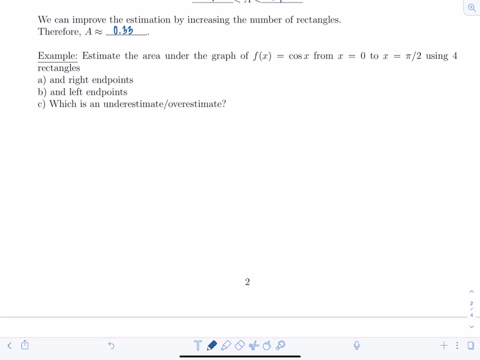 new function: instead of Y equals X squared. Let's move on And we're going to estimate the area underneath the graph of F of X equals cosine X, from X equals zero to pi over two, using four rectangles, And for the first part we're going to use right end points. For the second, 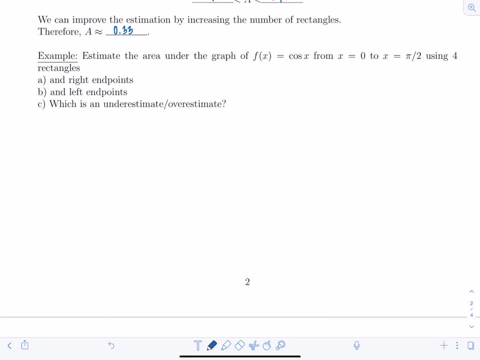 part, we're going to use left end points and then determine which one's an underestimate, which one's an overestimate. So to begin, we have to draw a picture. So for part eight, we're going to be using right end points. cosine of X from X equals zero to pi over two. 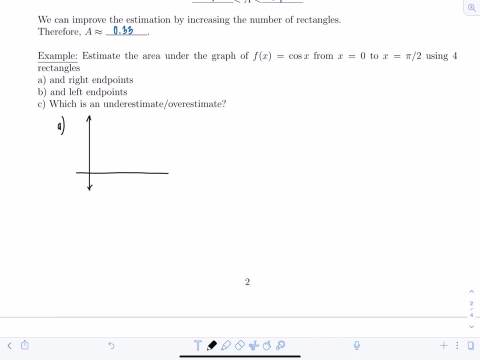 Well, we know, at zero, cosine is equal to one, And then we're only going up to pi over two. Here's my X axis, And we're using four rectangles, right, Four rectangles. So here's how you want to think of it. If your interval is from zero to pi over two, then each of the bases 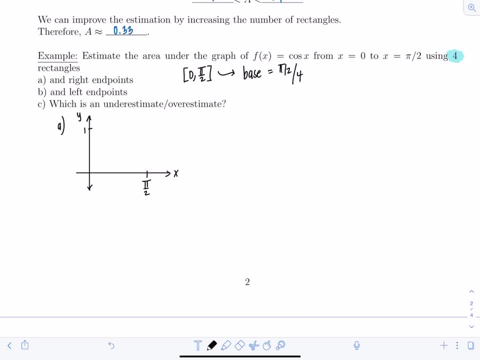 is going to equal pi over two divided by four right, Which would be pi over eight. So that would be the length of each of the sub intervals. So here I'm going to cut it in half, That's at pi over four, Cut it in half again, That's pi over eight, And then cut it in half one more time. 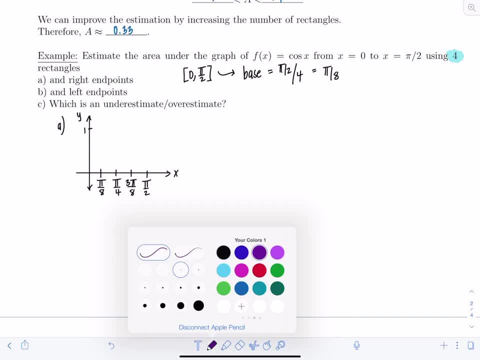 That's three pi over eight, Okay. And you don't have to draw a super perfect graph, Just know that cosine X is one when X is zero. And then it's zero at pi halves And it curves downwards, right, It's concave down, Okay. So for right endpoint estimate I would use for the interval from zero. 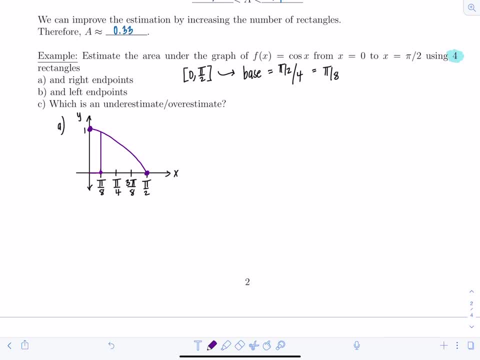 to pi eighths, pi eighths. That would be my first rectangle, That's A1.. For my second rectangle, I would use pi over four. For my third rectangle, I would use three pi over eight. That's A3.. 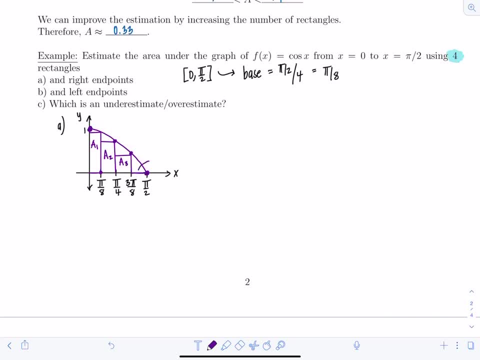 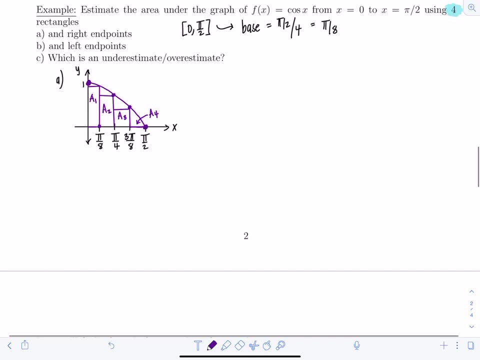 And for the fourth rectangle I would use pi over two. So you can't even see it, Okay, So let's list it out. So R4 is going to equal. Now notice: the base on each of these is pi over eight. It's equal, right? So I can just take pi over eight and then multiply by the. 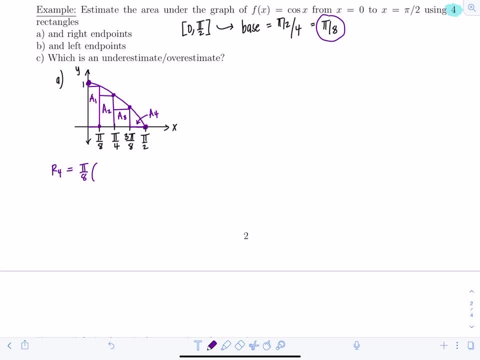 function heights at each of those four endpoints, the right endpoint So pi over eight, pi over eight, pi over four, three pi over eight and pi over two. So I have pi over eight times cosine of pi over eight, plus cosine of pi over four, plus cosine of three pi over eight, plus cosine of pi over two. 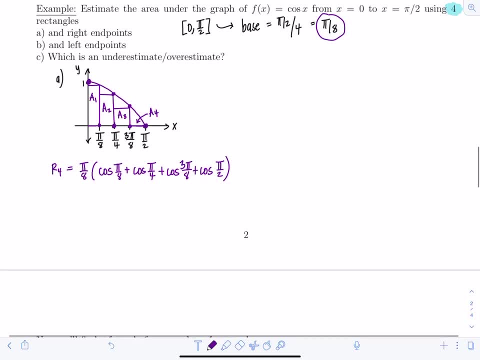 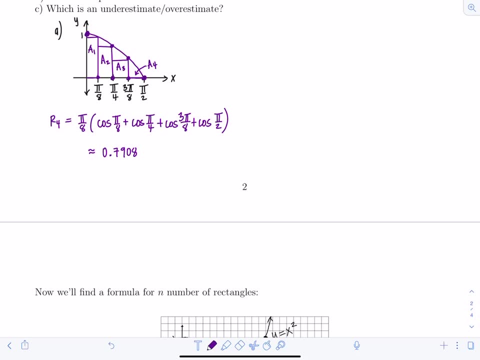 All right, And then you could substitute all these in your calculator And we end up with approximately point seven nine zero eight for R4.. All right, now would you say this is an overestimate or an underestimate. Always use the graph to determine, okay. So notice, each of these rectangles lies. 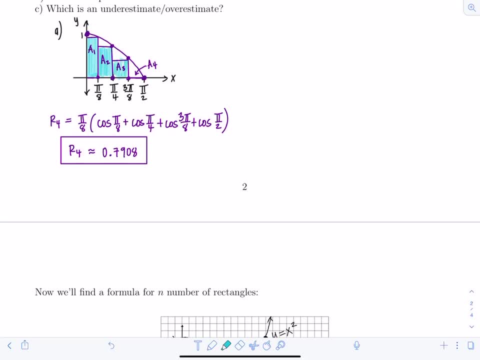 below the curve. So in this case, R4 is an underestimate. Now, in the previous example, with y equals x squared, R4 was an overestimate. So why is it different in this case? Well, it depends on the concavity of the curve that you're dealing with. Y equals x squared is concave. 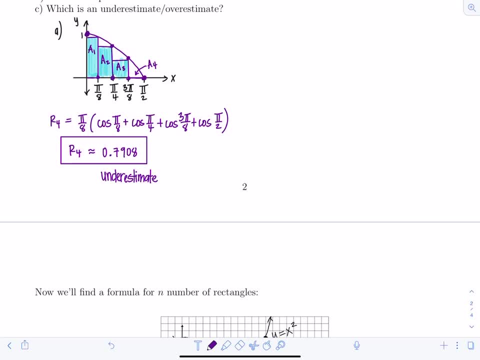 up, and in this case cosine of x is concave down on the interval from zero to pi over two. So don't memorize, but just use the graph to help you determine whether or not your approximation is an overestimate or an underestimate. All right, now let's perform the same estimation. 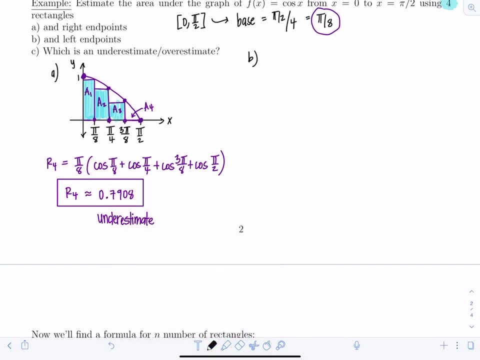 but this time we're going to use left-end points, So we're going to divide up the interval in the same way. so, from zero to pi over two, Here's one. here's pi over two. here's pi over four, pi over eight. three pi over eight. 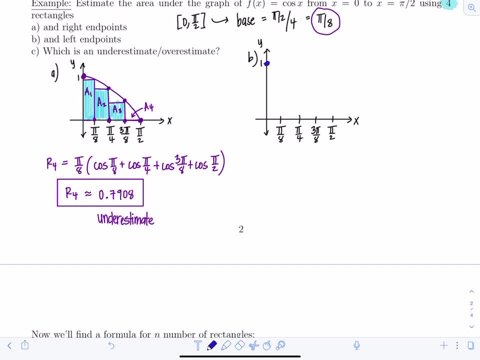 Cosine starts at one, goes to zero at pi over two, and this time I'm taking left-end points, So I'm going to use zero for the height of the first rectangle, That's a1.. I would use pi over four for the height of the second rectangle. 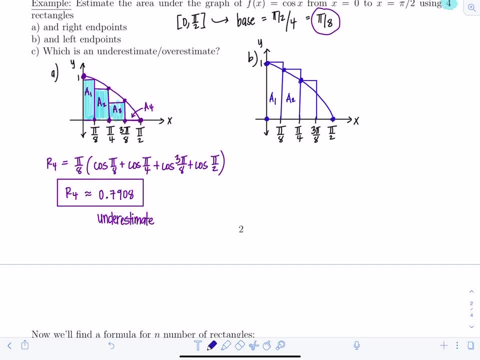 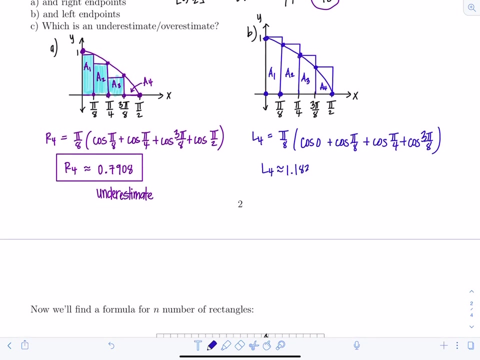 then pi over four, and then three pi over eight. Ok, Good, so L4 is equal to pi over ten, 8, and then I would have cosine of 0 plus cosine of pi over 8, plus cosine of pi over 4, plus cosine of 3 pi over 8, and l4 comes out to approximately 1.1835 all. 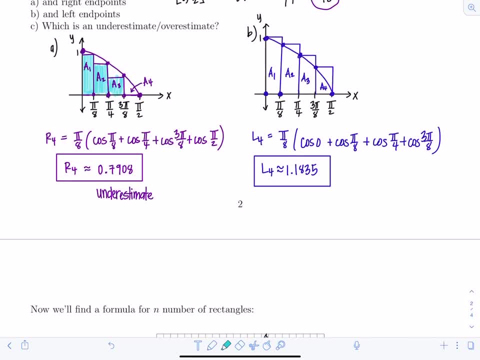 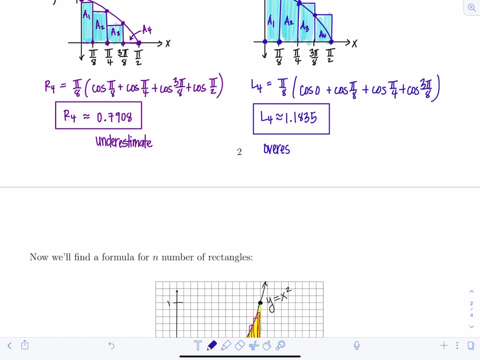 right. would you say this is an over estimate or an under estimate? remember, use the graph and look at these rectangles and you see how the height of each of them is a little bit above our curve, cosine X. well, that means then that it is an over estimate. okay, good. so, like we said before this, taking a finite 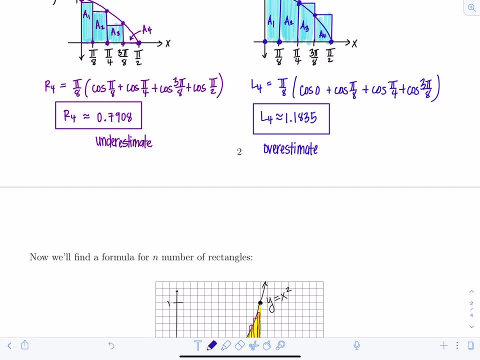 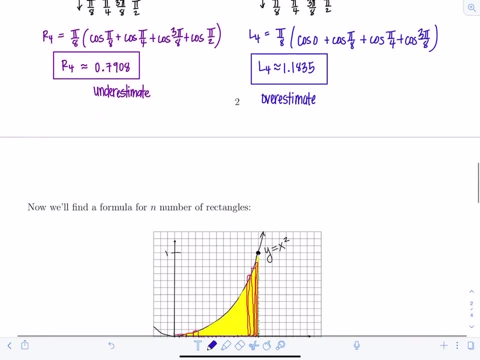 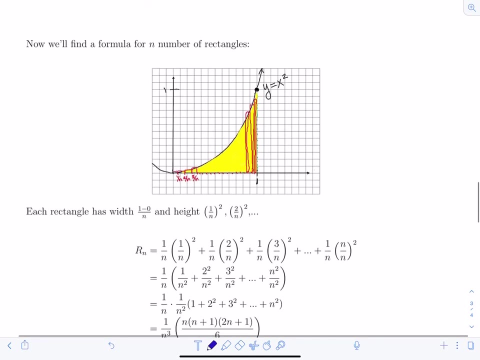 number of rectangles here gives us an approximation, but it's not an exact value for the area underneath the curve, and we're not happy about that. so what we want to do is improve our estimate, and now that we're in calculus, we can talk about things like infinitely many rectangles. so what I want to do is find 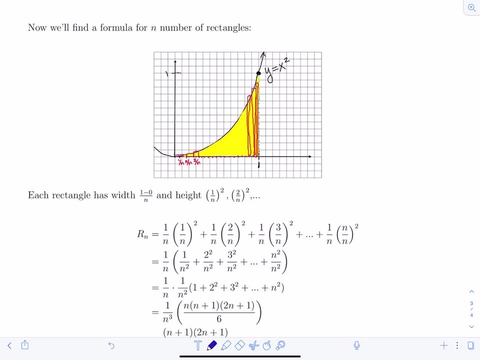 a formula for the area under the curve using n number of rectangles. so I'm gonna leave n as a variable, and then what we're gonna do is take the limit as n goes to infinity, because the more and more rectangles we use, the error starts approaching zero, and so we want to just 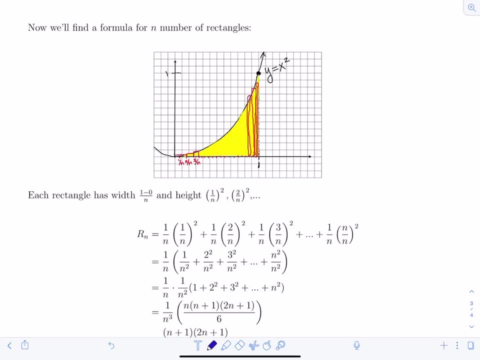 let n go off into infinity, so that we have no error left. okay, so we're gonna go back to our example of y equals x squared, because that function is really nice to work with. and if I had n many rectangles, the width or the base of each? 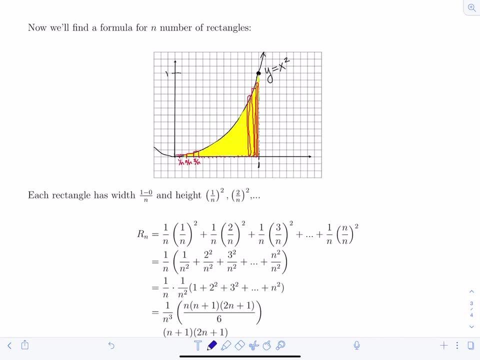 of them would be 1 minus 0 divided by n. well, where does that come from? well, it was just considering the area under the curve on the interval from 0 to 1 right, and last time, when we had four rectangles, we We took the length of that interval, which is one minus zero, and we divided by the number. 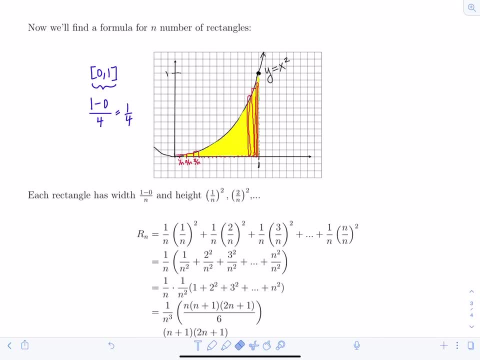 of rectangles, which was four, And that's how we got the base of one fourth. Well, this time we're saying we want to leave n as a variable and many rectangles, So the base of each of them would be one over n. 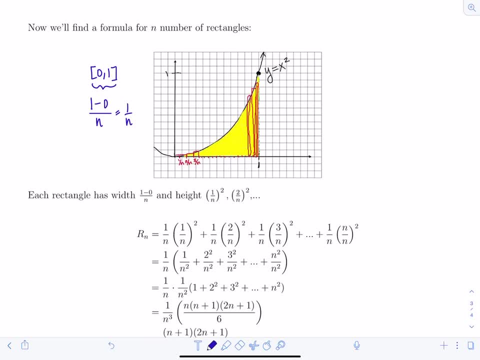 OK, and then the height, in this particular case, using right endpoints, would be one over n squared. If you zoom in here or I'll just draw the x-axis out separately, How about that? So here's your interval from zero to one right. 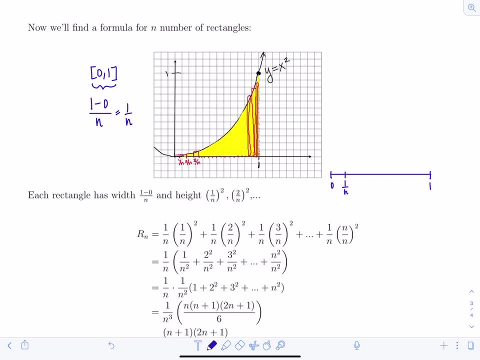 So the base of each of them is one over n. So that's one over n. Add another one over n. Now it's two over n. Add another one over n. It's three over n, et cetera, right. 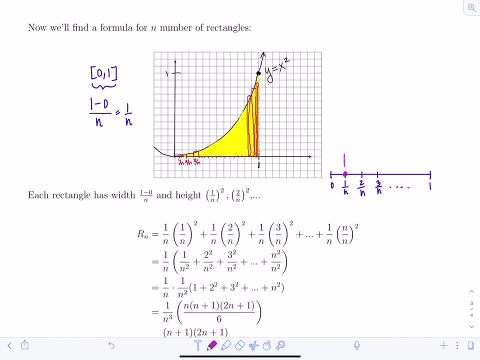 And if we're using right endpoints, then I'm going to evaluate the function here. So you would have f of one over n, f of two, Two over n, f of three over n. This is because we're taking right endpoints. 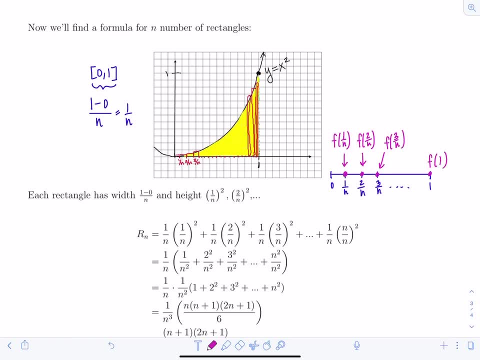 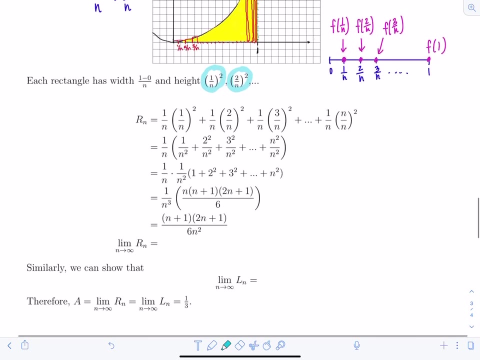 And then your last one would just be f of one, And our function here is x squared, which is why the height of each rectangle comes out to be one over n? squared, two over n? squared, so on and so forth. So my right endpoint approximation for n many rectangles is going to be one over n. 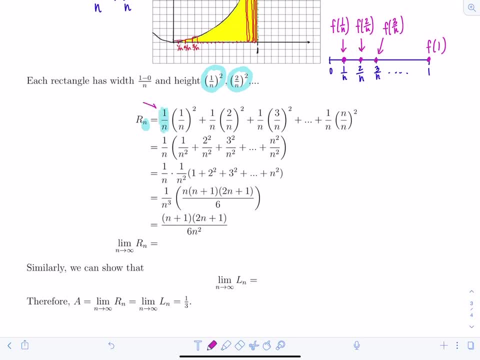 This is the base right, or the width, That's the width times the height, which is the function value, starting at one over n all the way up until n over n. That's the last one. And then notice, each of these have the same base of one over n, or the same width. 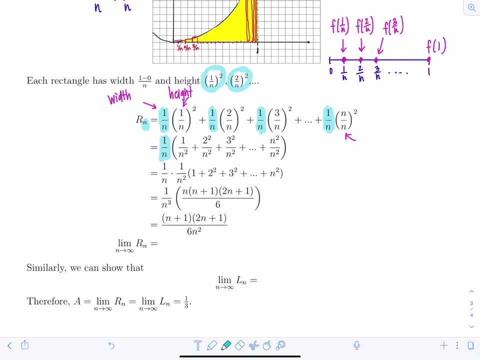 So I can factor that outside of the expression, just like we did in the previous example, how we factored out that pi over eight for cosine. Okay, And then all I'm left with is one over n squared two, squared over n squared three. 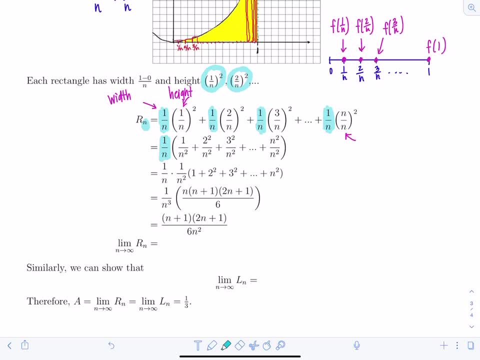 squared over n squared the sum of all those terms. Notice again, they all have n squared in common in the denominator, So I can factor that out as well. And then I'm just left with one over n times one over n squared times the sum one plus. 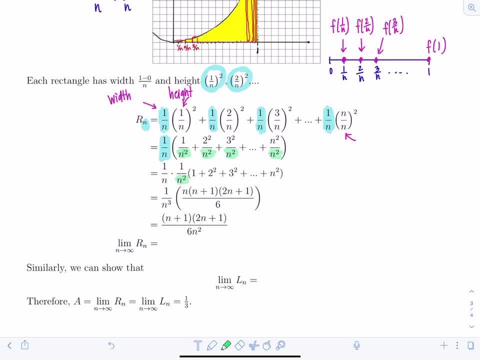 two squared plus three squared, plus dot, dot, dot, up until n squared. So we have one over n cubed sitting outside, And then we're going to study this more in the next section. but the sum one plus two squared plus three squared plus up until n squared we can replace with the following: 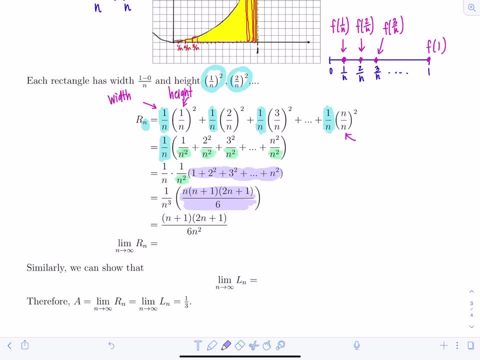 expression. Okay, That's more to come in section five, two. And then, simplifying from here, I can cancel out one of the n's here so that I just have n squared. So now we have six n squared in the denominator Okay. 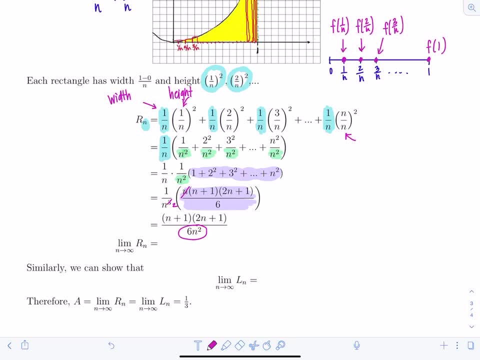 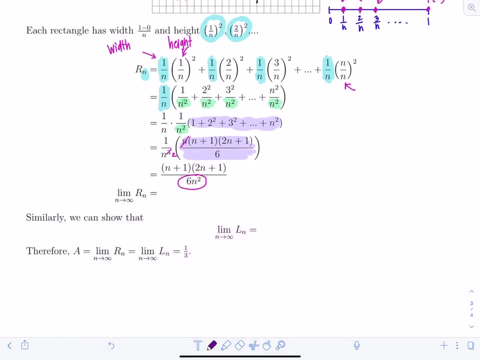 And then n plus one times two, n plus one. All right, So remember we said that as the number of rectangles increased, our error went to zero, And so we want to take the limit as n approaches infinity of r sub n, And this would equal the limit as n approaches infinity of two n squared. 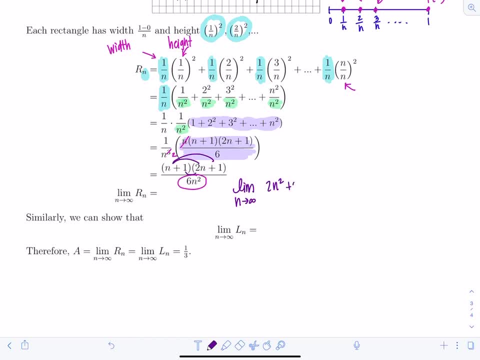 I'm just going to multiply out the numerator: plus three n, plus one over two n squared, Okay. Okay, Six n squared. And then, when I take this infinite limit degree of the numerator equals the degree of the denominator. So I can just divide the leading coefficients, and this is one third. 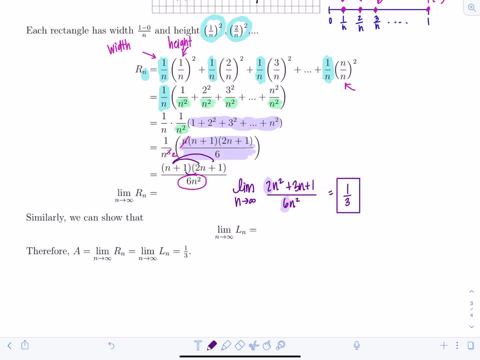 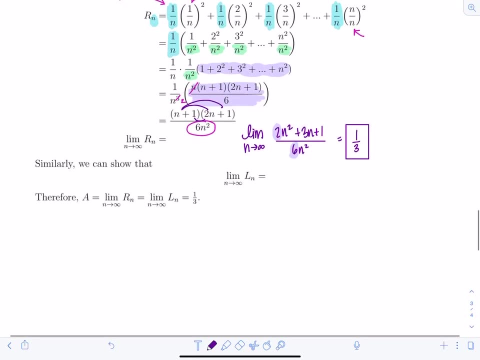 Okay, So we have, the limit as n approaches infinity of r sub n is one third, And similarly we can show that the limit as n approaches infinity of l sub n using left end points is also equal to one third. Ooh, very exciting. 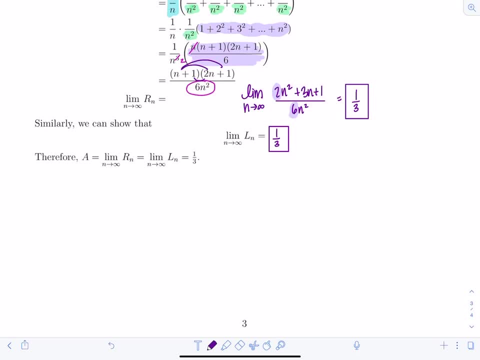 So therefore we have one third. Okay, So therefore we can say that the exact area underneath the curve y equals x squared on the interval from zero to one is equal to one third. So notice, I don't have any approximate. there's no error here. 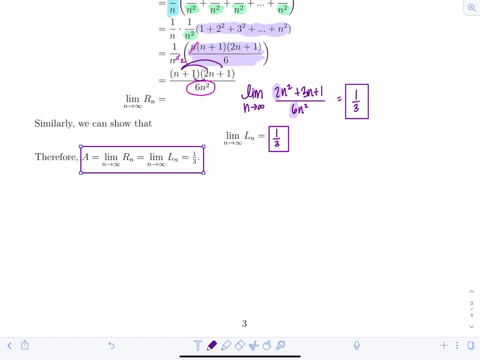 We know that it's exactly equal to one third. And notice that my right endpoint and left endpoint approximations are exactly equal to each other, because they're not approximations anymore. They represent the exact area under the curve. Okay, So that's the definition of the area under the graph of a continuous function f of x. 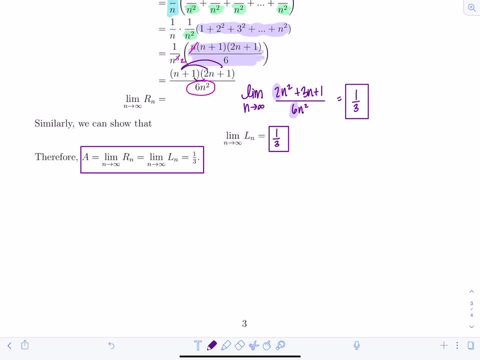 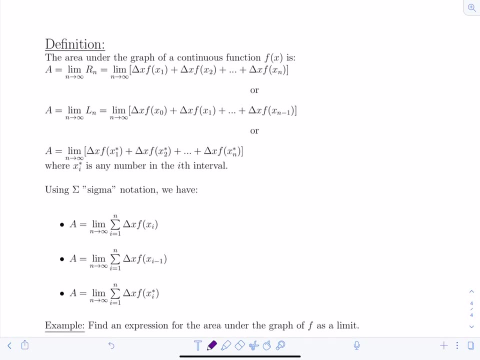 So the function has to be continuous- is equal to the limit as n approaches, infinity of r sub n. Remember that's the approximation used, taking right end points. Okay, So that's the definition of the area under the curve, which is the limit as n approaches. 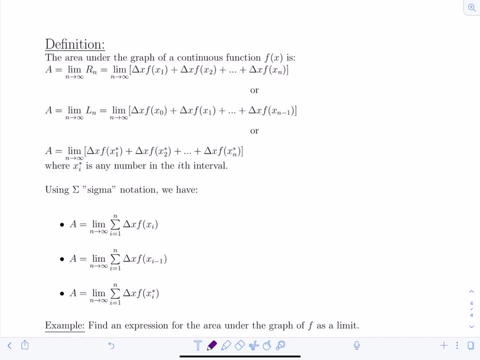 infinity of delta x times f of x1 plus delta x times f of x2, all the way up until delta x times f of xn. So delta x you could think of as your base. So that is the base of each rectangle or the width, okay. 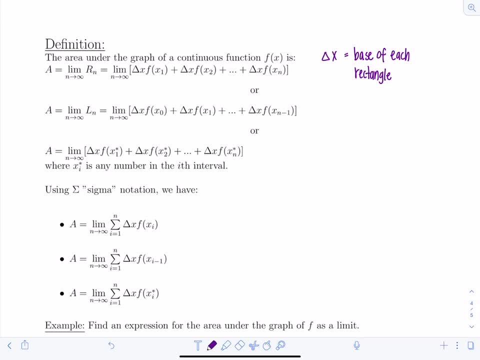 And if we're finding the area underneath the curve of a function on the interval from zero, from a to b, then in order to find delta x, you would take b minus a, the length of the interval, and then divide it by n. 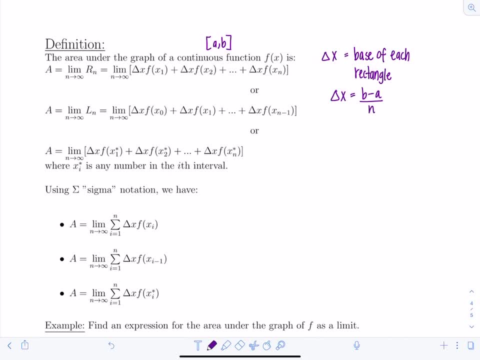 And then f of x1, f of x2, all the way up to f of xn. that's the function being evaluated at the right end points. Now notice the difference here if we're talking about left end points. My first function evaluation is at f of x0, and the last one is at f of x sub n minus. 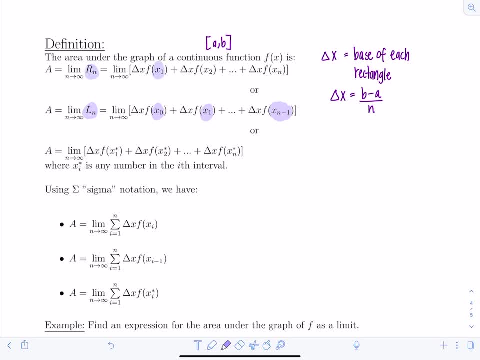 1, right. So you have to find the right end point and then, at f of x1,, all of those points are left end points. So if you're using the left end points versus right end points, you start at x1.. 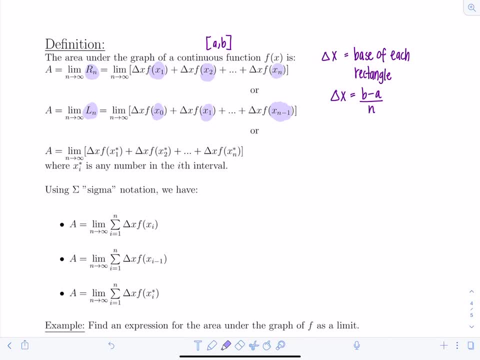 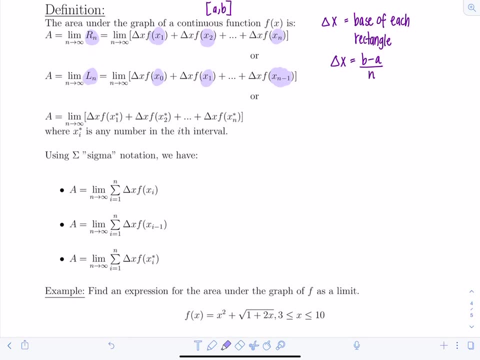 Also, who's to stop us to only use the left and right end points? We can use any function value on each of those sub-intervals and that's why sometimes you'll see a star represented, if it's not necessarily left or right. 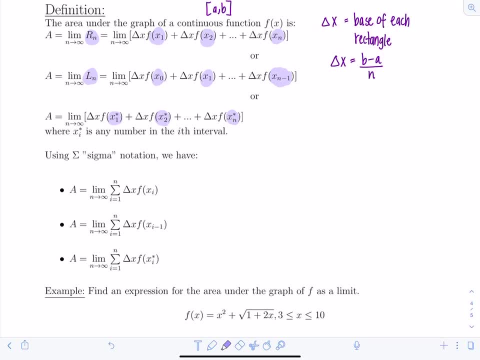 So f of x1 star, x2 star, up until xn star. Sometimes you use the midpoint Or sometimes you might take some other value to evaluate the function. so x sub i, sub n minus 1.. star is any number on the ith interval. Notice these all give you the exact area underneath the 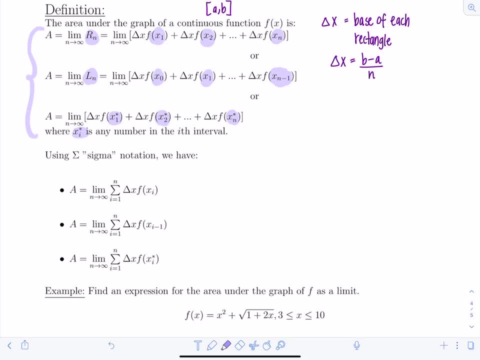 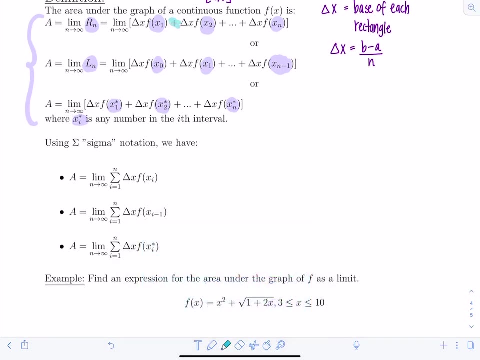 curve once you take that limit, as n approaches infinity, And as long as your function is continuous, it means it's going to be integrable, and so all of these limits will have the same value. All right now, using sigma notation right, who wants to write out the sum over and over? and? 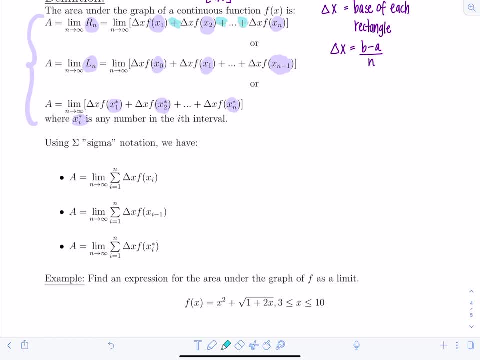 over. I can just replace it and write the limit as n approaches infinity, so that stays the same, and then we have the sum. i equals 1 to n of delta, x times f of x sub i. That's for right endpoints, The next one is for left endpoints and the last one is for some arbitrary partition. 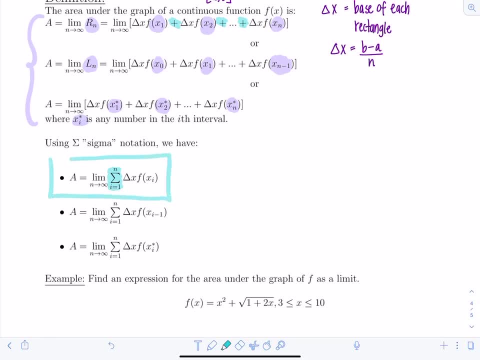 So the one we're going to work with in this class is the right endpoint version of the formula, just because it's the nicest to work with, since we just start from 1 and go up until 1.. n And we know that they all come out to be the same, So there's no need to work with all three. 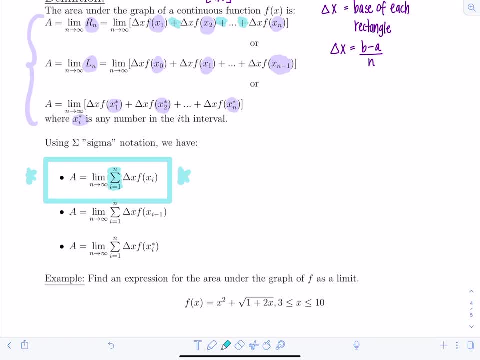 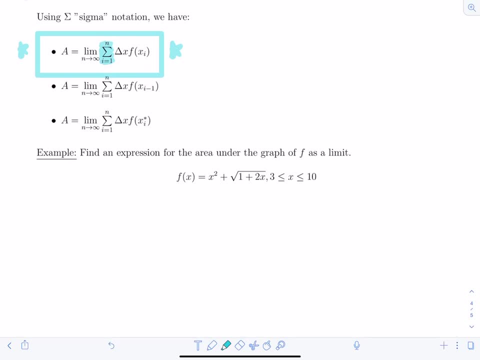 formulas necessarily at this point in your calculus career. Okay, good, So find an expression for the area under the graph of f as a limit. So basically, we just want to use this definition and expression in sigma notation to find an expression for the area underneath the graph. 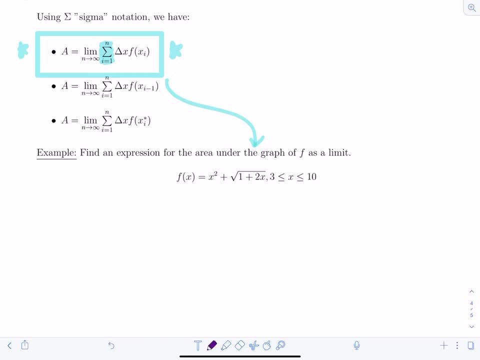 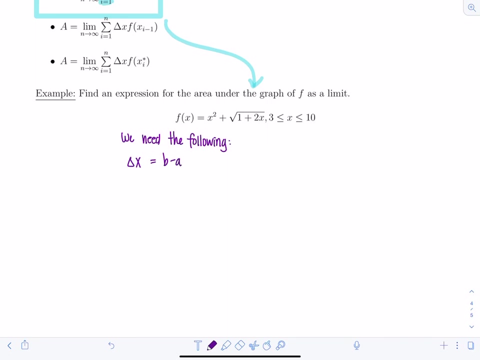 of the following function. So to build it we need to start with the following. So we need our delta x right, the base of each of them. So delta x is equal to b minus a over n. In this case there's a, there's b, So this is going to be 10 minus 3 over n, which is 7.. 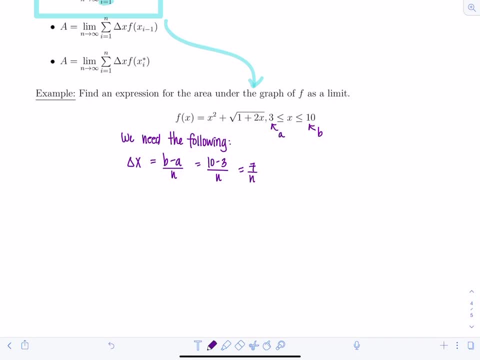 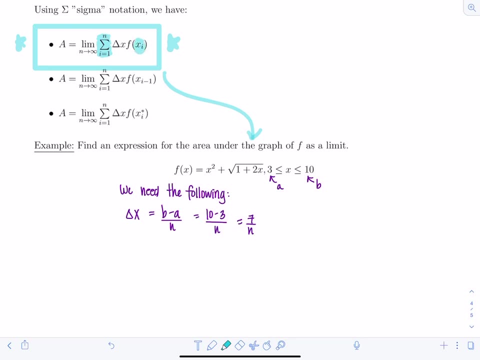 Over n. All right, looks good. Now. the next part of the formula involves f of x sub i. Well, what's x sub i? All right, let's draw out our interval here, Okay, and it's from 3 up until 10,. 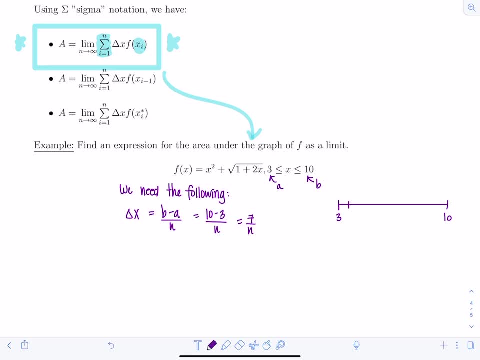 right. So each delta x is going to be the base of the rectangle, so on and so forth. So this is a delta x, this is a delta x, this is a delta x. And remember, we're using right endpoints to evaluate our function. So that would mean, on this first subinterval, I would take the height. 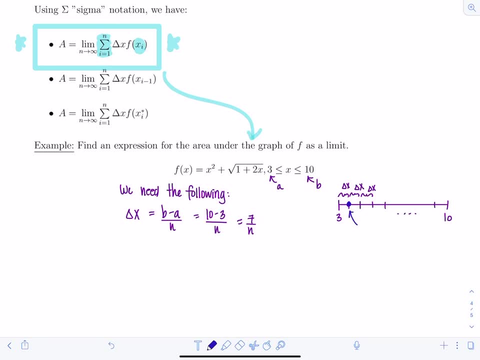 of the rectangle by plugging in whatever value for x that is. Well, what is that? That's 3 plus delta x. right, That's x1.. Okay, What about the delta x? Well, that's x1.. And what about this next one here for my second rectangle, That's x2.. Well, x2 would equal 3 plus. 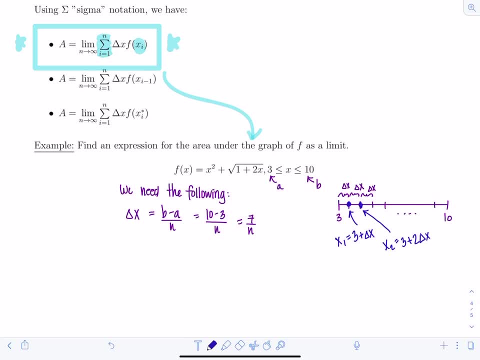 2 delta x's. And if I wanted an expression for x sub i right my i's subinterval, then that would be 3 plus i times delta x. Okay, So if you want an arbitrary formula for x sub i, general formula. 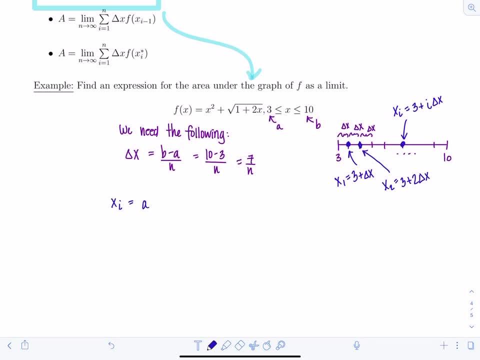 x sub. i would be a right, whatever the start of your interval is. In this case we started at 3 plus i times delta x, So in our case it's 3 plus i times there's delta x 7 over n. 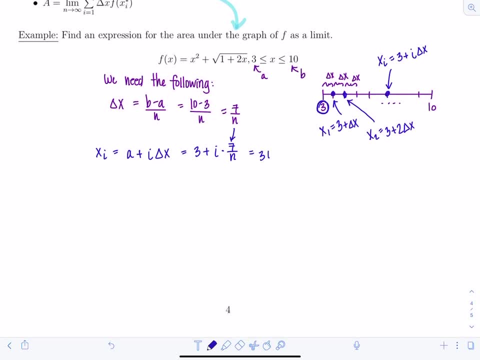 And then we can just clean that up and write it as 3 plus 7i over n. So this is always the order that you want to do it in. You want to find delta x, first x sub i and then you want to find delta x. 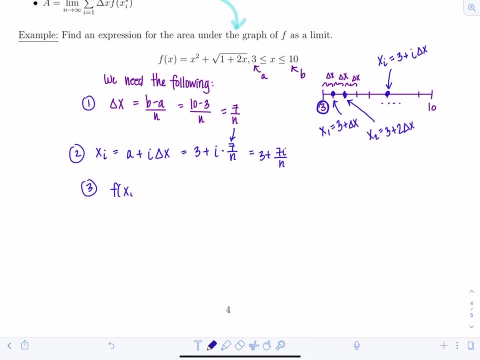 next. And then lastly f of x sub i. So I'm going to substitute 3 plus 7i over n into the function. So this is going to be 3 plus 7i over n, squared plus radical 1 plus 2 times 3 plus 7i. 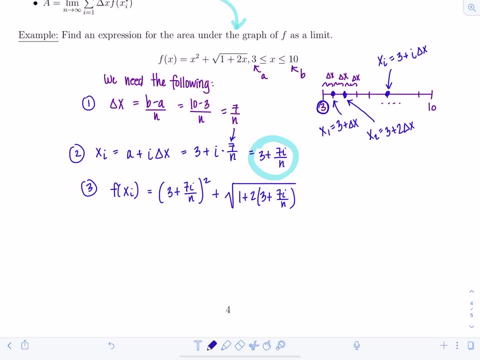 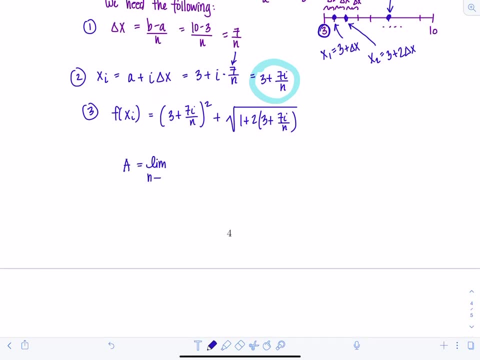 over n. Okay, So now we're going to put everything together. So the exact area underneath the curve equals the limit As n approaches infinity. remember that makes our error go to zero. I'm adding up all the rectangles. I start at i equals 1.. I end at n. 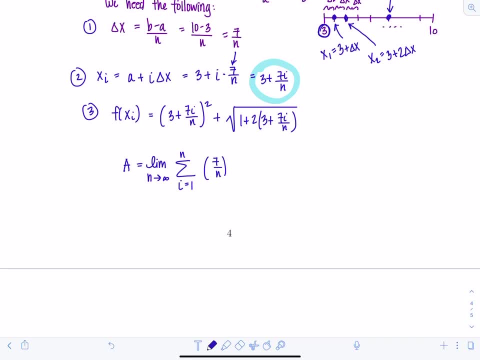 I have the base of each rectangle. Base is 7 over n, or the width times the height, the function value, which is going to be 3 plus 7i over n squared, plus radical, And then we will clean this up a little bit- That's 6i over n squared. So we're going to put everything together. 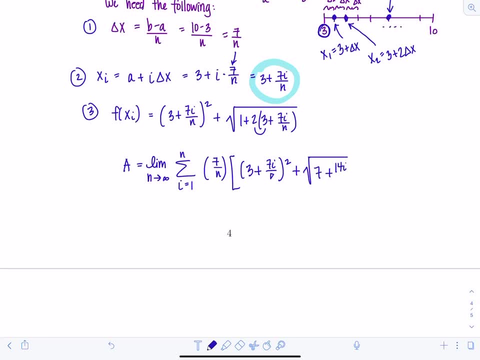 6 plus 1 is 7 plus 14i over n. What happened to this guy? Okay, This is an n And that's our final answer. We're not going to evaluate this limit, Don't worry, That's for the next. 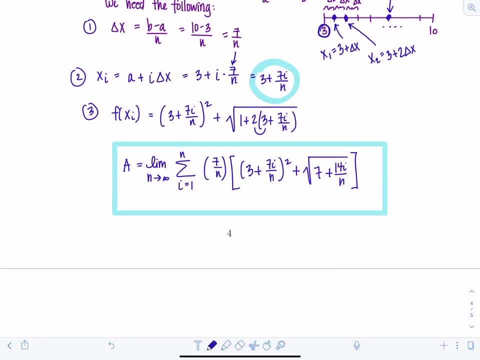 lesson, But when you're building this, I want you to think of it this way: This is the base or the width, This is the height for each rectangle. We add them all up, And then this makes our error go to zero. 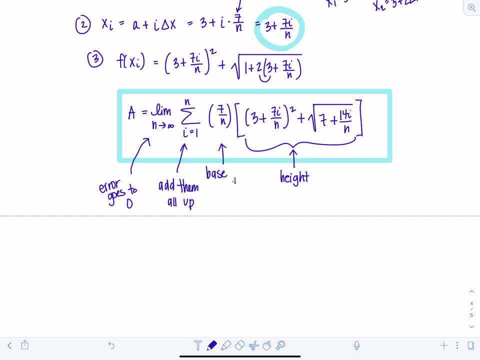 And if you think of it that way, then the formula won't seem so arbitrary. All right, So that concludes the lesson. Hope you enjoyed it And then stay tuned for the next video, because we're going to actually evaluate this limit for various kinds of functions. Thanks for watching. 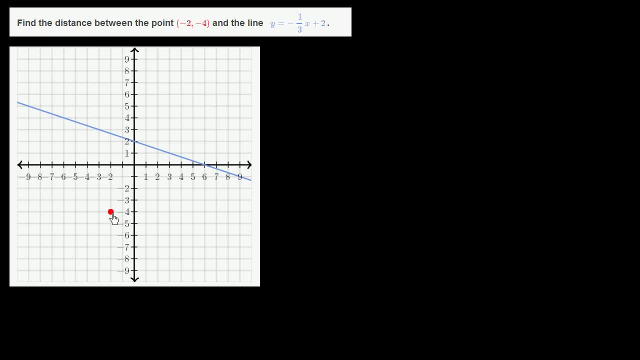 Find the distance between the point negative 2, negative 4, this point right here and the line y is equal to negative 1, third x plus 2.. That's this line right over here. Now to do it, we just need to figure out. 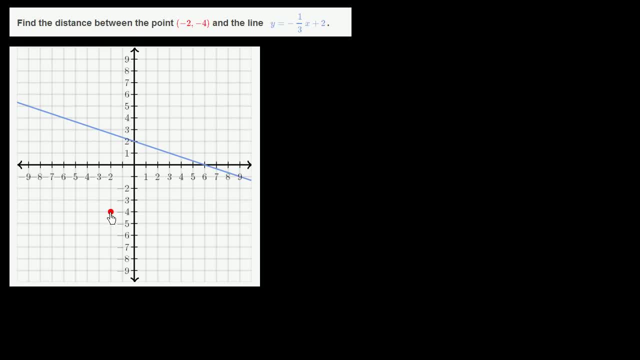 a perpendicular line to this blue line to y is equal to negative 1 third x plus 2, that contains this point right over here. So we need to figure out the equation of this line and then we need to figure out where do these two lines. 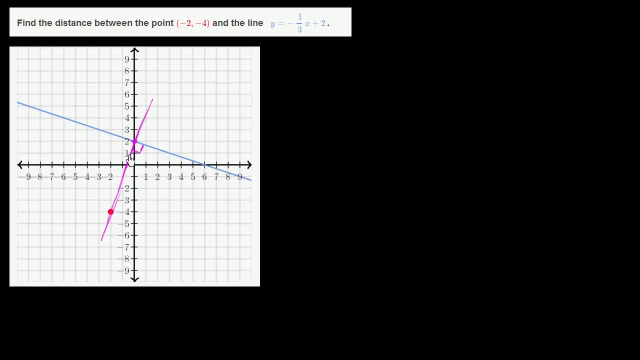 intersect, and then we need to find the distance between these two points of intersection, And we have the shortest distance between this point and this line right over here. So the first step is to figure out what is the slope of this perpendicular line. Well, the slope of a perpendicular line